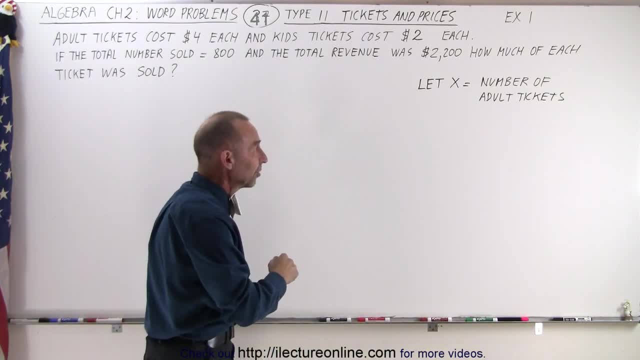 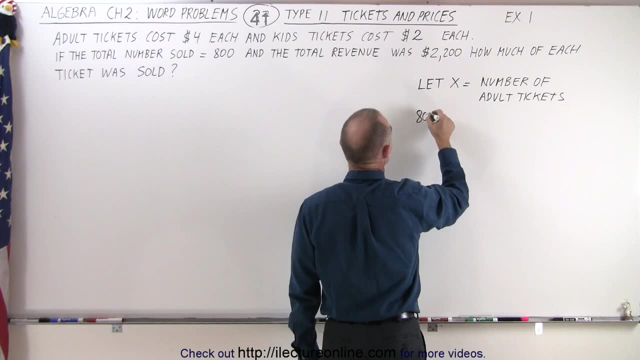 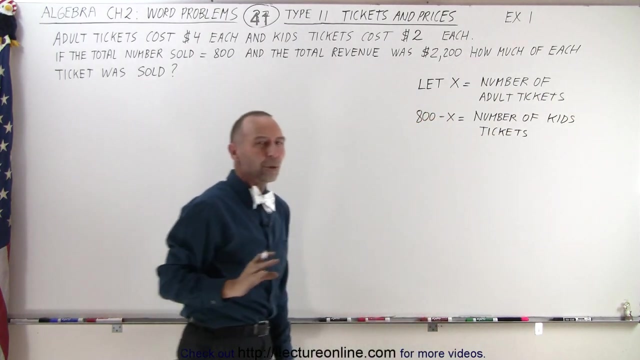 of 800 were sold, then 800 minus x should be the remainder of the tickets, which in this case would be kids tickets. So 800 minus x equal the number of kids tickets. Now we're going to need an equation to solve this problem. We're told that the total revenue was 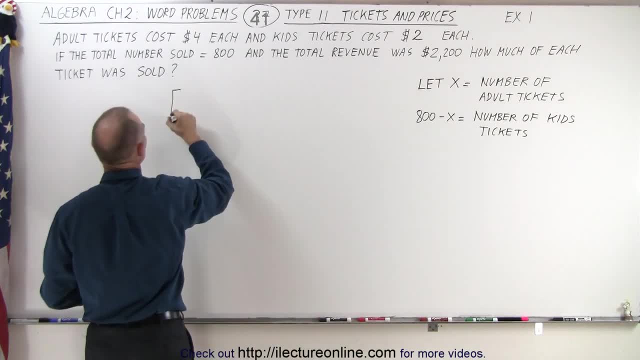 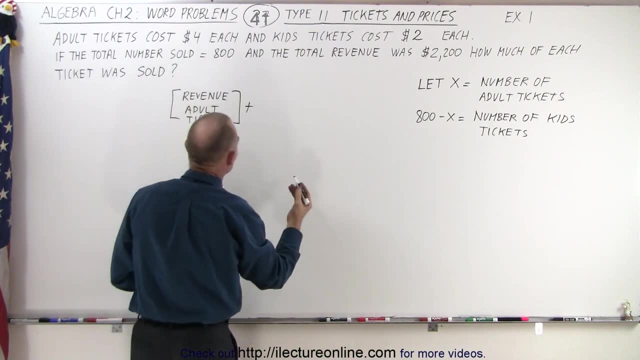 $2,200,, which means that the revenue that we took in for the adult tickets plus the revenue that we took in for the kids tickets together should add up to the total revenue received. Now we have an equation. Now we just have to simply put that into practice, And we're going to need an equation to 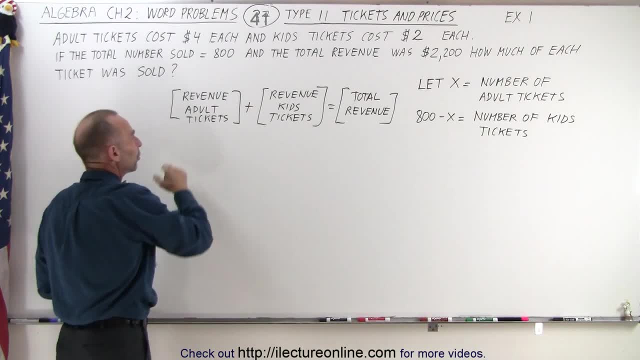 solve this problem. So the revenue of adult tickets would equal the amount that each ticket cost times the number of tickets that we sold. So each ticket cost $4 and the number of tickets sold was x. So four times x $4, for each ticket times the number of adult tickets, gives us the revenue for all the 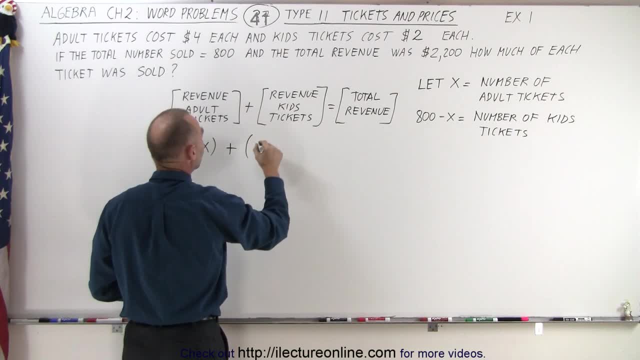 adult tickets The same for the kids tickets. $2 for each ticket times the number of kids tickets, which in this case is 800 minus x The amount for each ticket times the number of tickets sold. That will be the revenue for the kids. 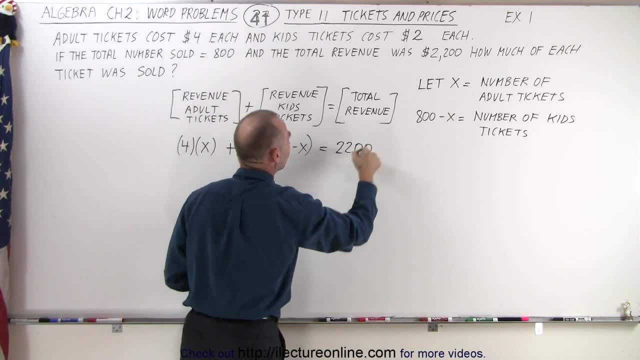 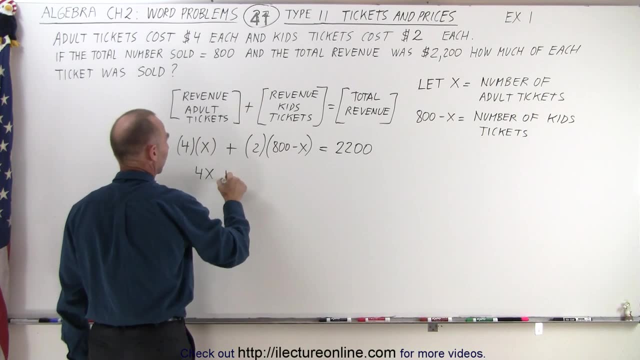 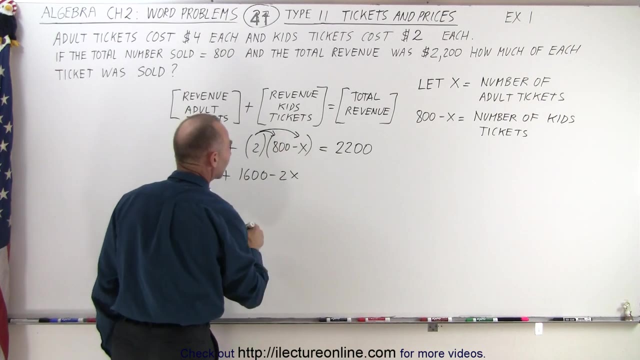 tickets and the total revenue is equal to $2,200.. We're now ready to solve this for x. First we get rid of the parentheses: $4x plus $1,600 minus $2x As we distribute the $2 on both the $800 and the x, and that adds up to $2,200, bring the $1,600. 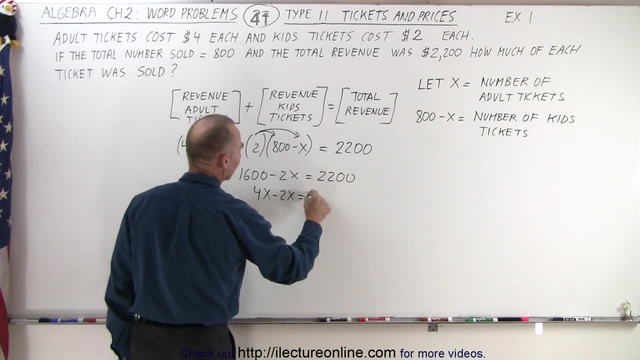 across $4x plus $2,200.. $4x plus $2,200: bring the $2,200 across $4x. bring the $1,600 across andование to llhe $2,200.. minus 2x is equal to 2200 minus 1600. when we bring the 1600 to the other side becomes minus 1600. 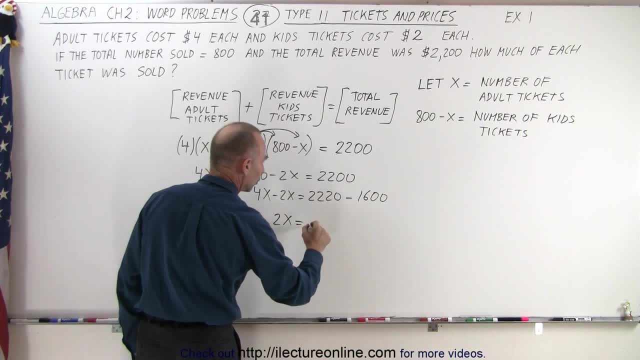 4 minus 2 is 2x is equal to. let's see here that would be- oh, I have one too many twos. that should be a zero. that would be 2200 minus 1600, which is 600, and therefore, when we divide both sides by 2,